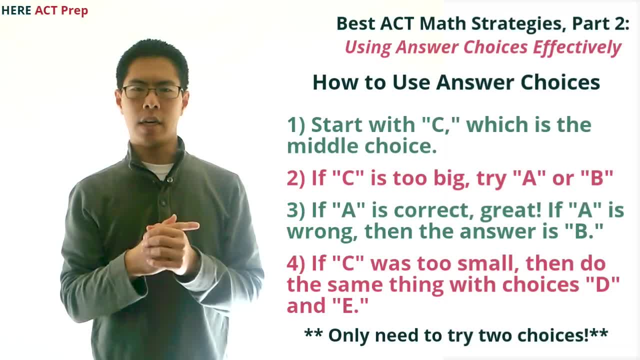 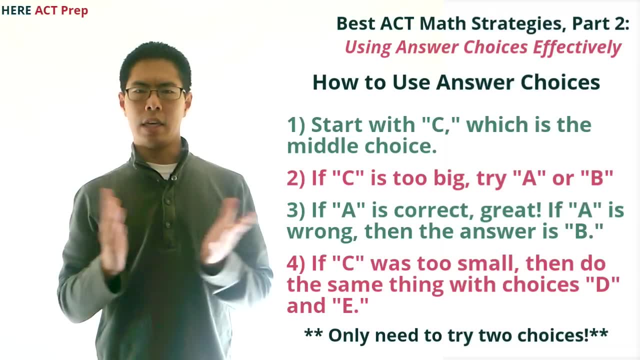 in. If it's right, then great. If it's wrong, then we know the answer is the other one. Likewise, if C ends up being too small, then we know the answer will be either D or E, so we pick one of them to plug in. 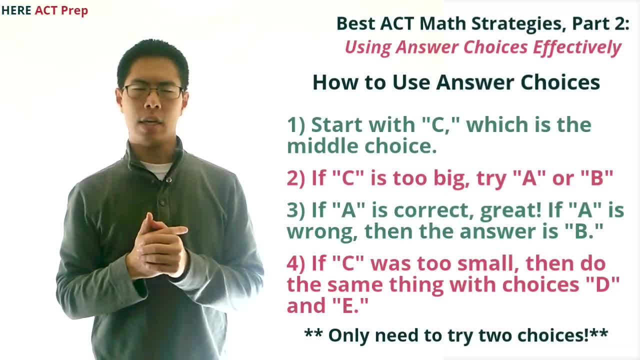 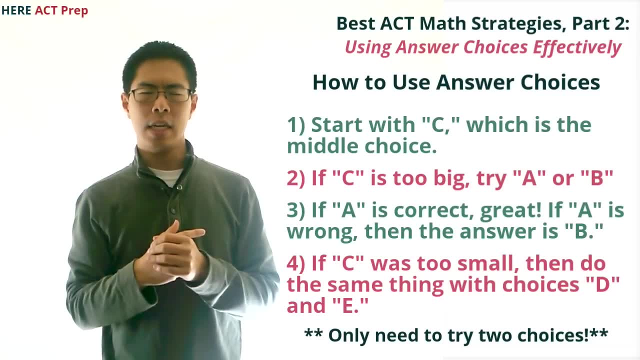 If it's right, great. If it's wrong, then we know the answer is the other one. On the other hand, if we just started with choice A and worked forwards, we might need to try four different choices if the answer is E, instead of just two, using this method. 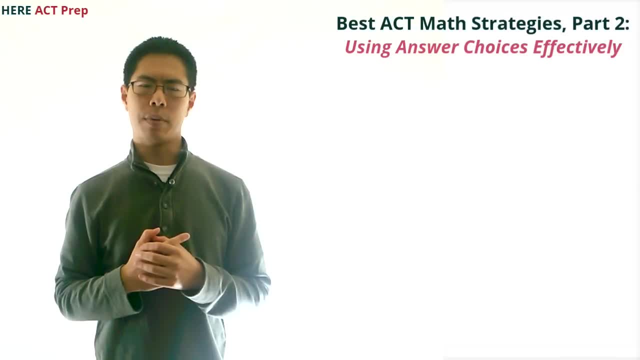 where we start with C. Now let's try this with two examples. First, let's take a look at this question: If 2n plus 1 squared minus n minus 5 squared, equals 16, then what could be a value of n? 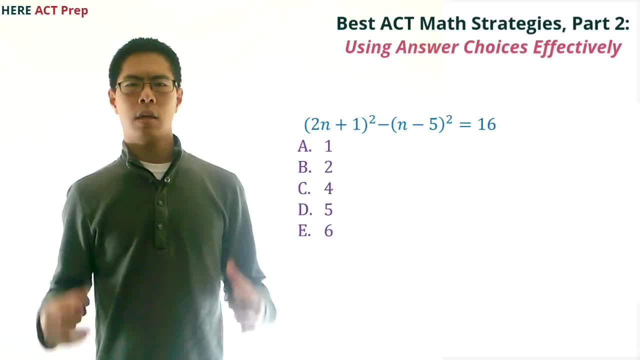 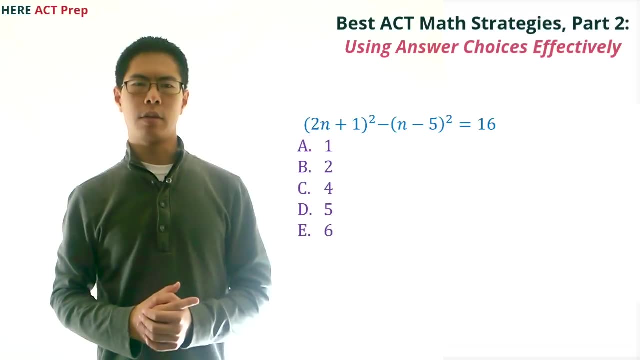 Our choices are 1,, 2,, 4,, 5, and 6.. For this question, we should recognize that it would take quite a while to FOIL out the entire problem and find the roots, so this would be a perfect question to use the answer. 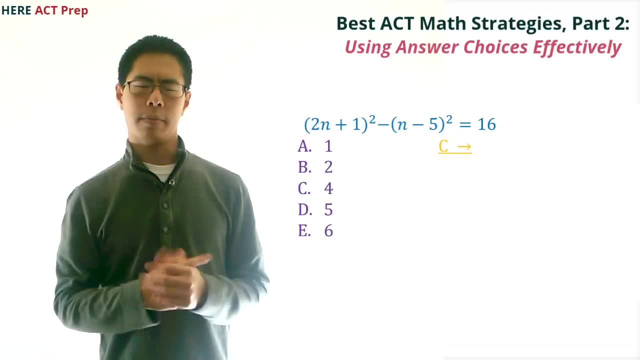 choices for. So let's start by trying choice C, which is 4.. When we plug 4 in, we end up getting 9 squared minus negative. 1 squared equals 16, which simplifies to 81. minus 1 equals 16,, which is 80.. 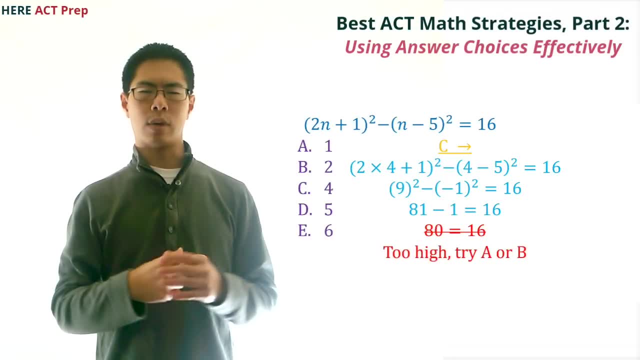 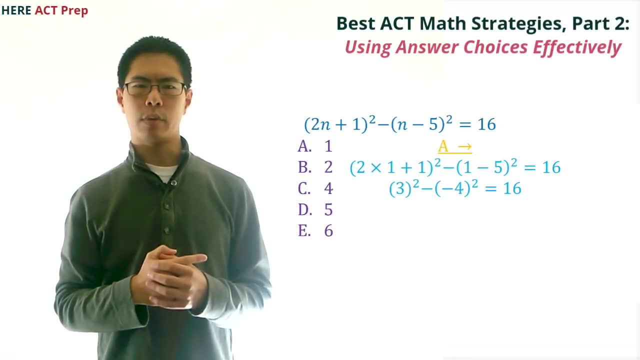 Okay, We see that 80 is too big, so let's try one of the smaller choices. Let's try A by plugging 1 back into the original equation. When we do this, we end up getting 3 squared minus negative. 4 squared equals 16, which. 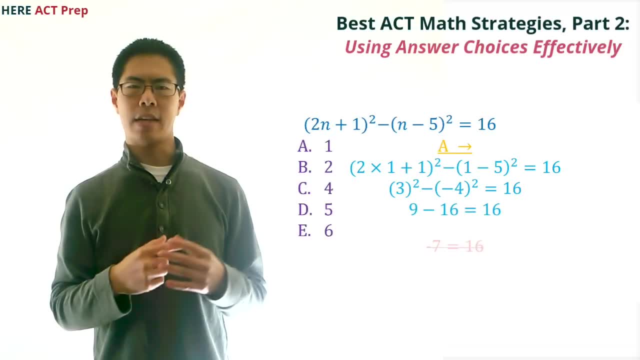 simplifies to 9 minus 16 equals 16,. which simplifies to negative, 7 equals 16,, which doesn't work either. So now we know the answer needs to be between A and C or between 1 and 4, so we can just. 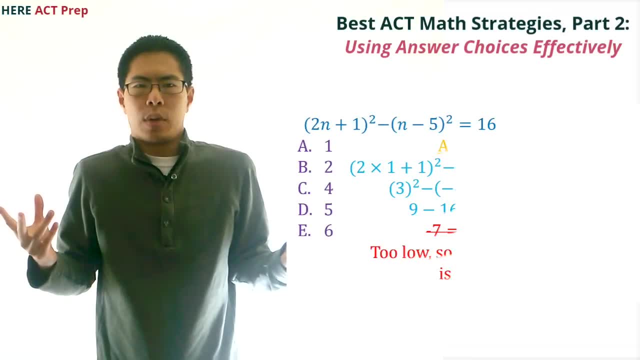 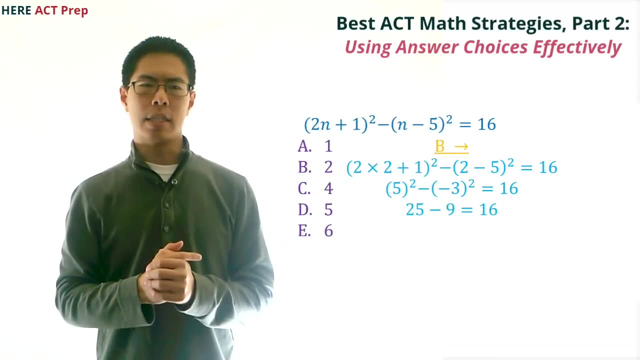 pick B at this point and move on. But if we wanted to check this, we would see that plugging 2 back into the equation gets us 5 squared minus negative, 3 squared equals 16.. So we end up getting 3 squared equals 16, which simplifies to: 25 minus 9 equals 16,. 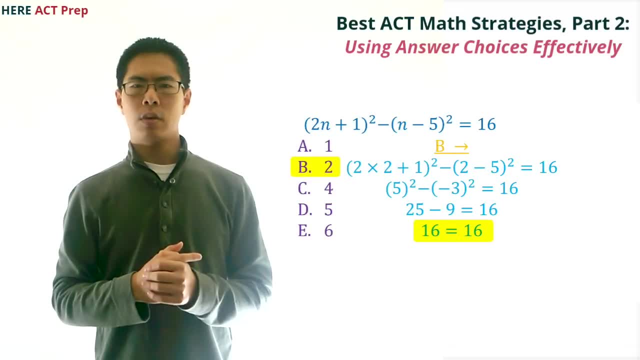 which simplifies to 16, equals 16.. With this method of using the answers, we will only need to try at most 2 of the answer choices, whereas if we started from the beginning we might need to try up to 4 choices. 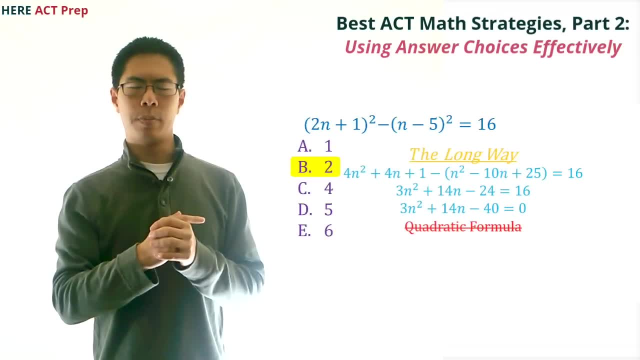 Now, if we wanted to actually set this question up and solve it, we would have had to distribute or FOIL out everything, combine all the like terms, get everything to one side so they equal 0, and then find the roots, probably using the quadratic formula, which would have: 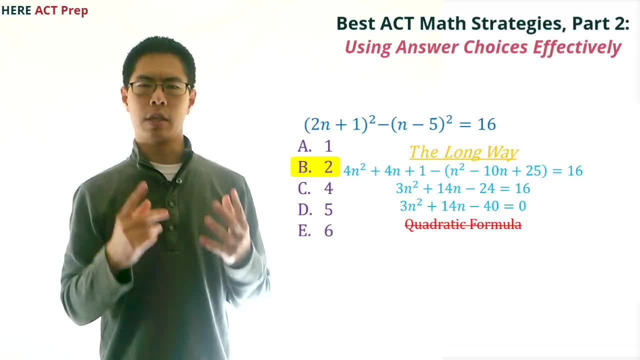 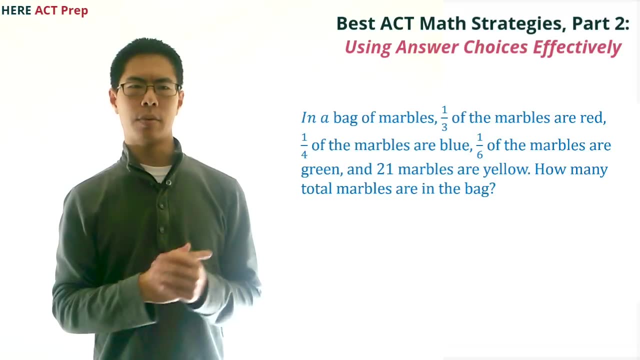 taken a lot longer. Using the answer choices was a much better idea. Now let's try one more example together. Let's take a look at this question. In a bag of marbles, one third of the marbles are red. one fourth of the marbles are blue. 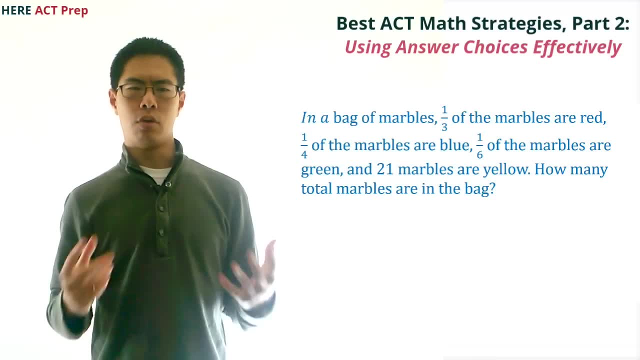 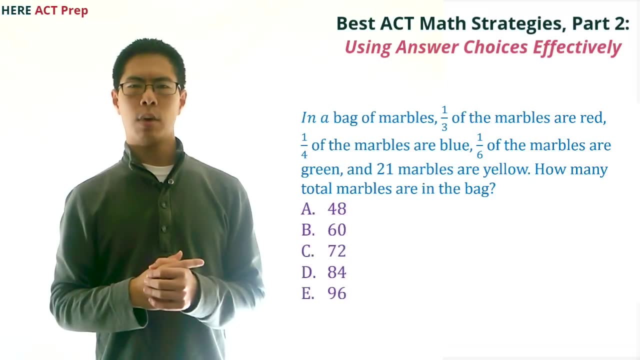 one sixth of the marbles are green and 21 marbles are yellow. How many total marbles are in the bag? Our choices are 48,, 60,, 72,, 84, and 96.. Like with the last question, we can figure out pretty quickly that this question will. 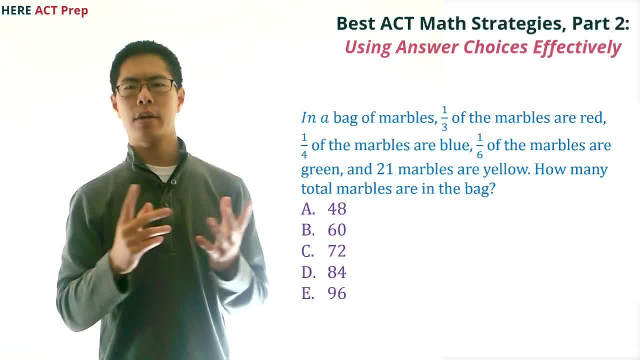 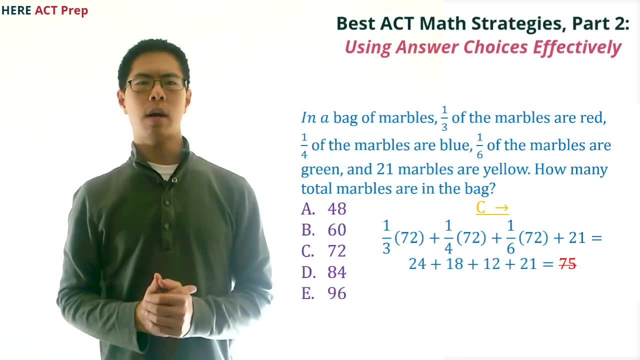 take a while to set up and solve and that using the answer choices will probably be quicker and easier. So here's how we could use the answer choices. Let's start with C, which is 72.. If there are 72 marbles in the bag, then one third or 24, are red, one fourth or 18,. 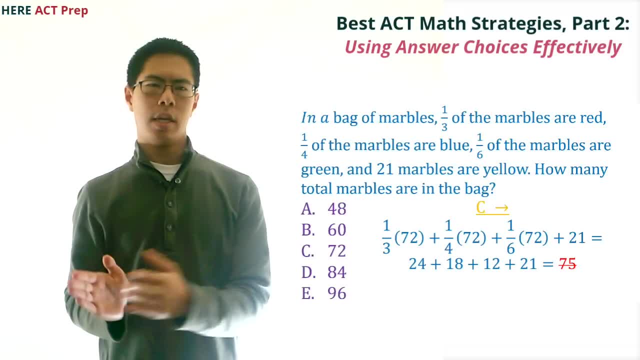 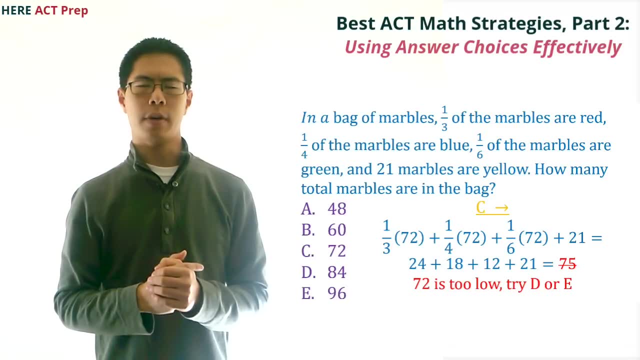 are blue. one sixth or 12, are green and 21 are yellow. This adds up to 75 marbles, which is higher than 72, so we know that 72 is too small, which means we should try D or E for our next answer. choice to use. 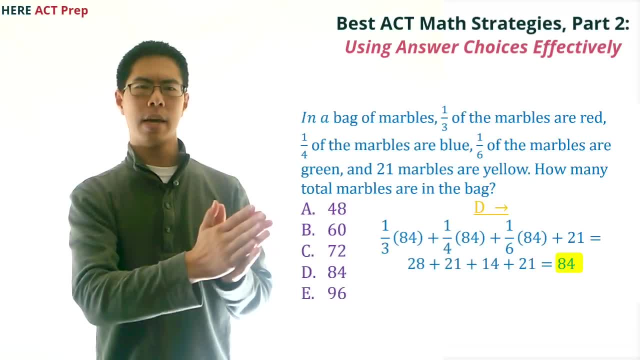 Let's try D or 84. If there are 84 total marbles in the bag, then one third, or 28,, are red, one fourth, or 21,, are blue, one sixth or 14, are green and 21 are yellow. 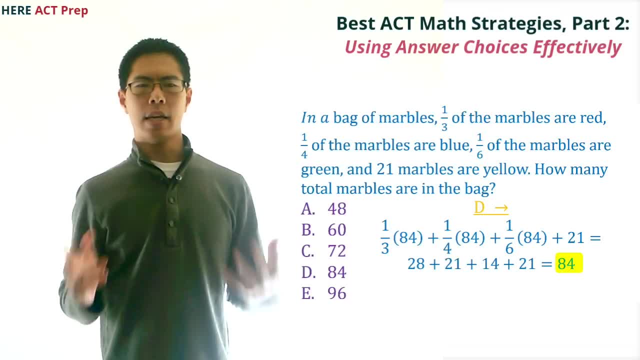 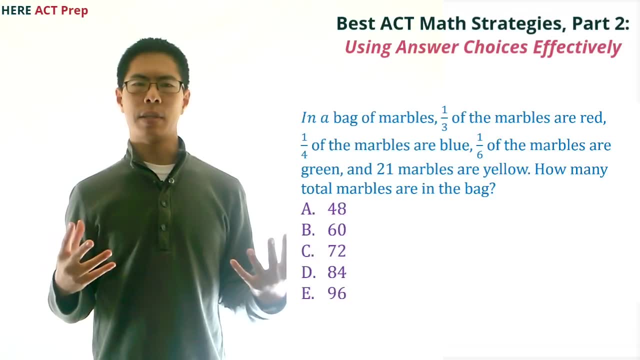 This adds up to 84, which is what we were aiming for. so our answer is D. As you can see, if we had started from A and moved forward, we would have needed to try three answer choices instead of just two. If we had wanted to set up and solve an equation for this question, we would have done one. 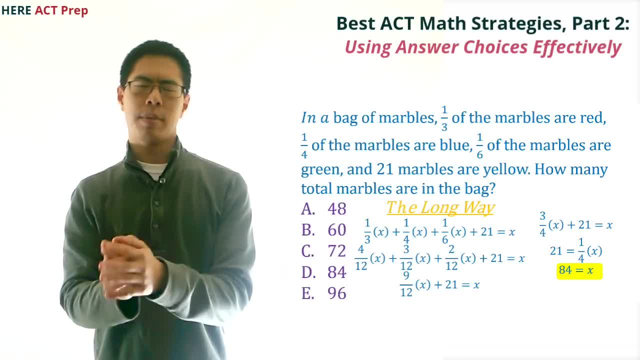 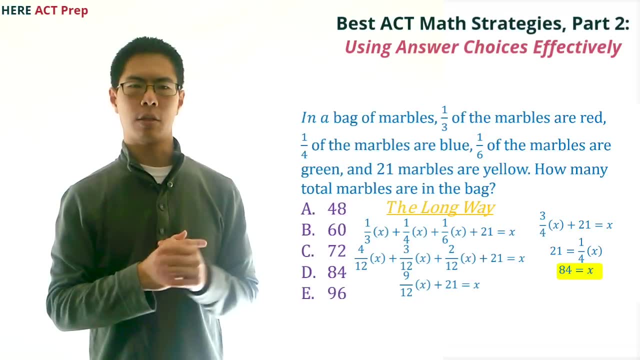 third x plus one. fourth x plus one. sixth x plus 21 equals x. then we would have changed the fractions to common denominators to get 4 over 12 x plus 3 over 12 x plus 2 over. 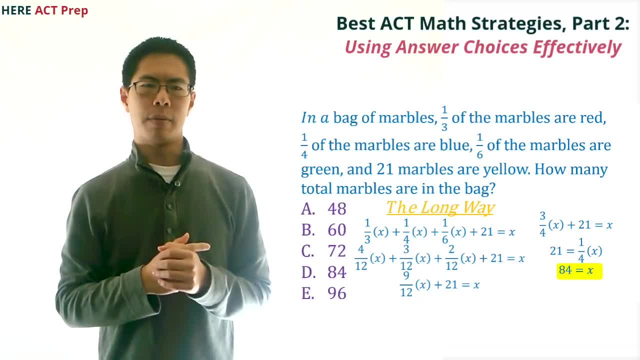 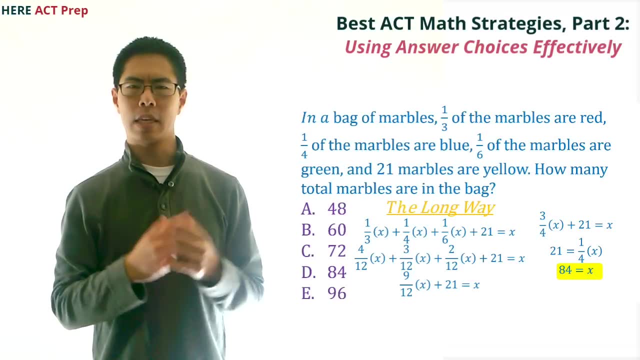 12 x plus 21 equals x. then we would have combined the like terms to get 9 over 12 x plus 21 equals x, which simplifies to 3 over 4 x plus 21 equals x. then we subtract 3. 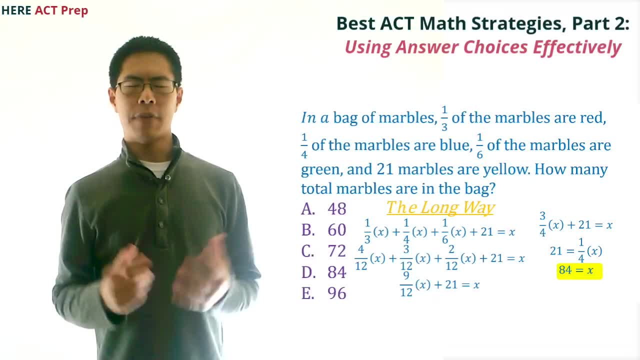 over 4 x from both sides to get 21 equals 1 over 4 x. and finally, we multiply both sides by 4 to get x equals 84, which is our answer. but that took a lot longer than just using the answer choices. 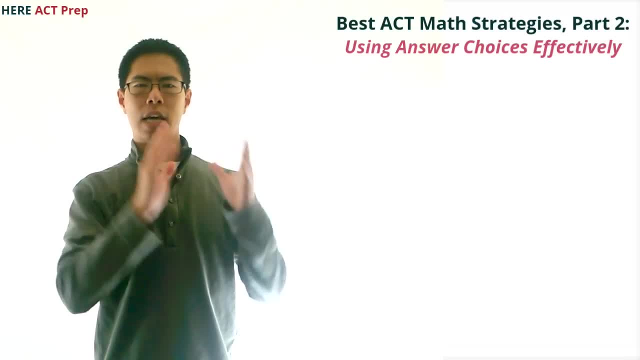 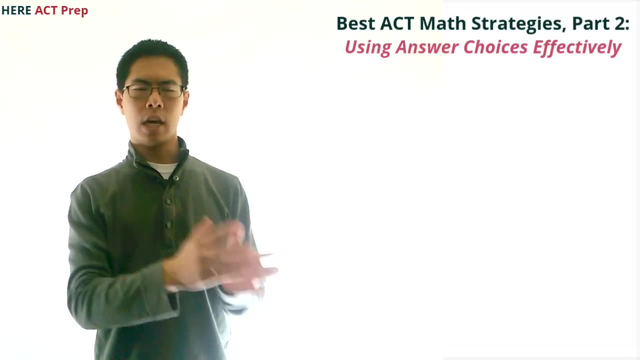 So the two examples that we just went through helped give us an idea of what kinds of questions would be good candidates for using the answer choices. Generally speaking, the questions that we want to consider using this method for are ones we're setting up, and solving the algebraic equation would take longer than just plugging.